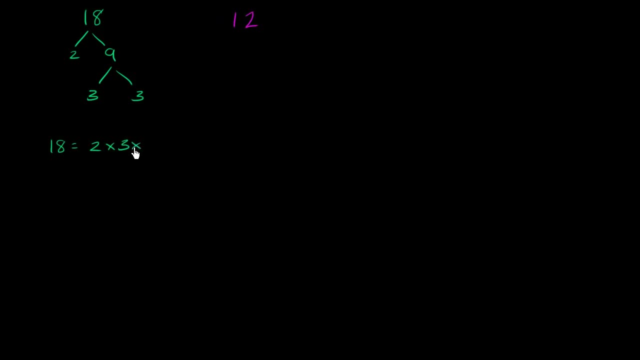 So we could write: 18 is equal to 2 times 3 times 3.. That's its prime factorization. 12 is 2 times 6.. 6 is 2 times 3.. So 12 is equal to 2 times 2 times 3.. 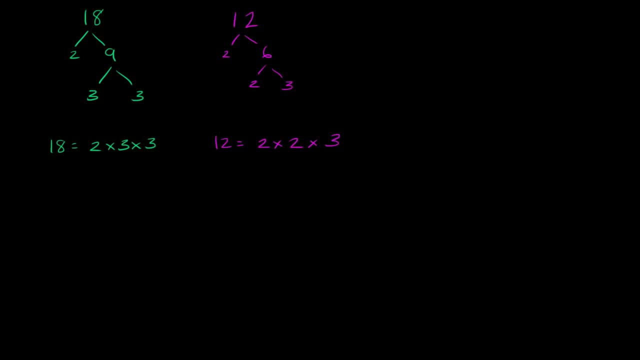 Now the least common multiple of 18 and 12, let me write this down. So the least common multiple of 18 and 12 is going to have to have Enough prime factors to cover both of these numbers And no more, because we want the least common multiple. 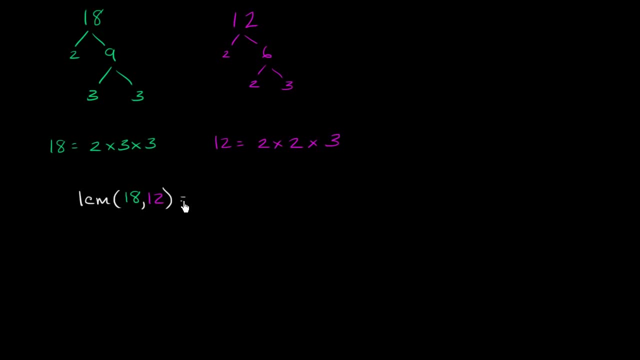 or the smallest common multiple. So let's think about it. Well, it needs to have at least 1,, 2,, a 3, and a 3 in order to be divisible by 18.. So let's write that down. 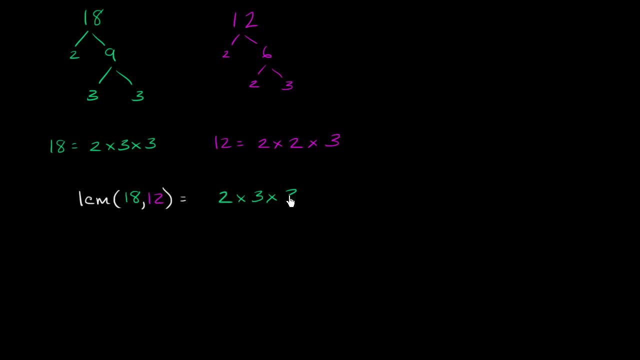 So we have to have a 2 times 3 times 3. This makes it divisible by 18. If you multiply this out, you actually get 18.. And now let's look at the 12. So this part right over here, let me make it clear. 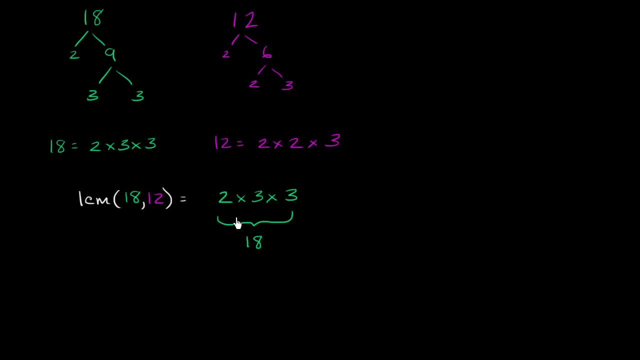 This part right over here is the part that makes up 18,, makes it divisible by 18.. And then let's see 12, we need two 2's and a 3.. Well, we already have one 3, so our 3 is taken care of. 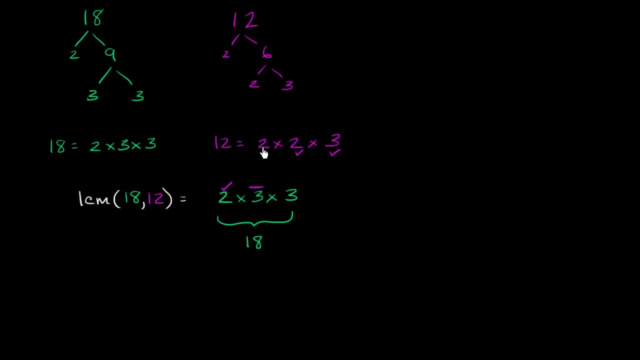 We have one 2,, so this 2 is taken care of, But we don't have two 2's, so we need another 2 here. So notice now: this number right over here has a 2 times 2 times 3 in it, or it has a 12 in it. 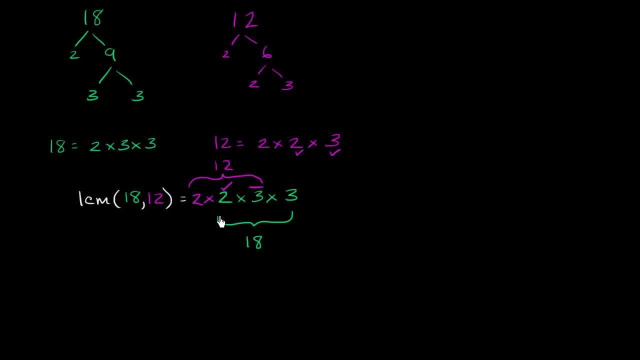 And it has a 2 times 3 times 3, or an 18 in it. So this right over here is the least common multiple of 18 and 12.. If we multiply it out, so 2 times 2 is 4.. 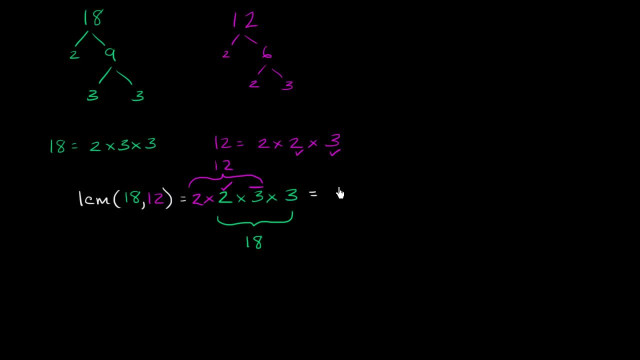 4 times 3 is 12.. 12 times 3 is equal to 36.. And we are done Now. the other way you could have done it is what I would say, just the brute force method of just looking at the multiples of these numbers. 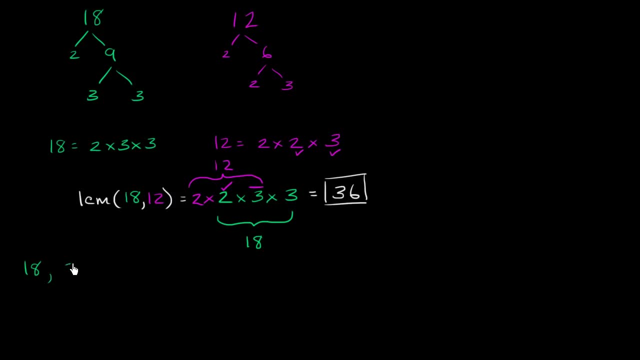 You would say: well, let's see, the multiples of 18 are 18,, 36,, and I could keep going higher and higher, 54. And I could keep going, And the multiples of 12 are 12,, 24,, 36.. 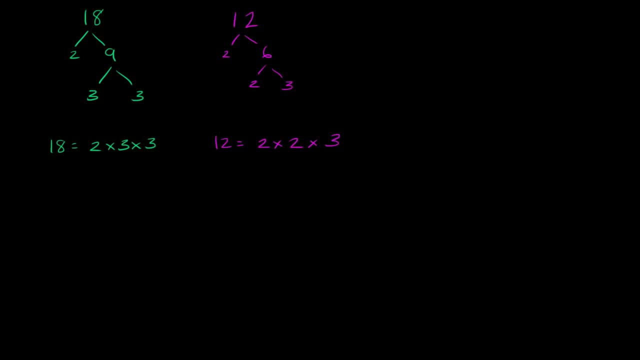 Now the least common multiple of 18 and 12, let me write this down. So the least common multiple of 18 and 12 is going to have to have Enough prime factors to cover both of these numbers And no more, because we want the least common multiple. 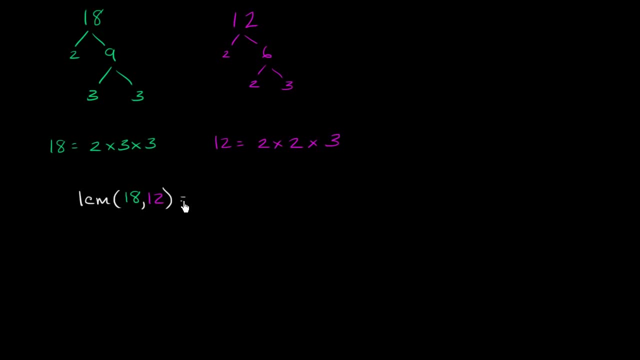 or the smallest common multiple. So let's think about it. Well, it needs to have at least 1,, 2,, a 3, and a 3 in order to be divisible by 18.. So let's write that down. 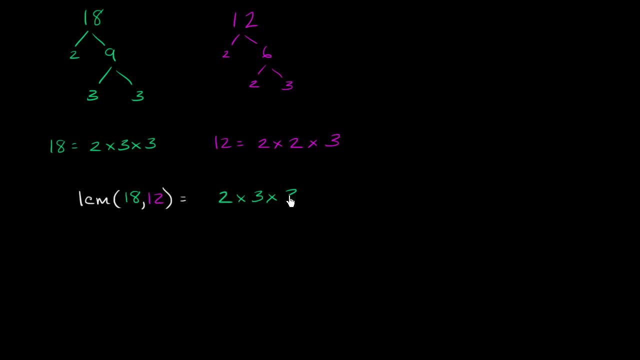 So we have to have a 2 times 3 times 3. This makes it divisible by 18. If you multiply this out, you actually get 18.. And now let's look at the 12. So this part right over here, let me make it clear. 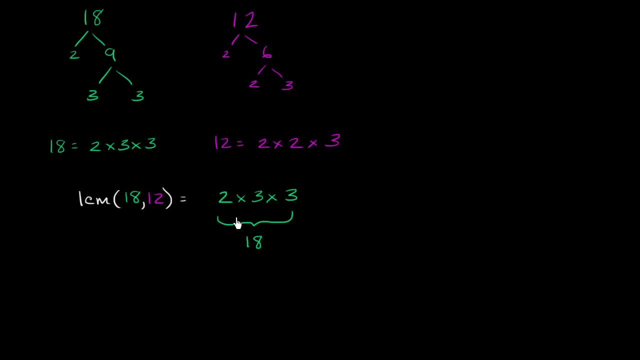 This part right over here is the part that makes up 18,, makes it divisible by 18.. And then let's see 12, we need two 2's and a 3.. Well, we already have one 3, so our 3 is taken care of. 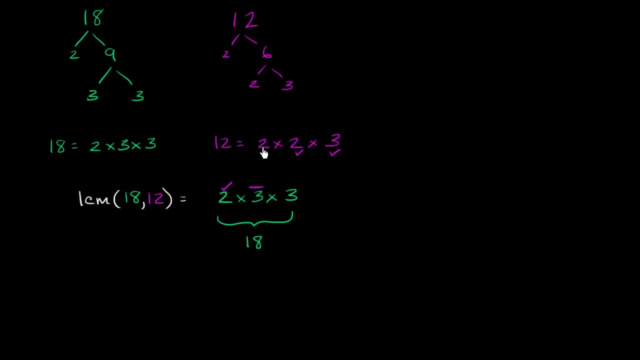 We have one 2,, so this 2 is taken care of, But we don't have two 2's, so we need another 2 here. So notice now: this number right over here has a 2 times 2 times 3 in it, or it has a 12 in it. 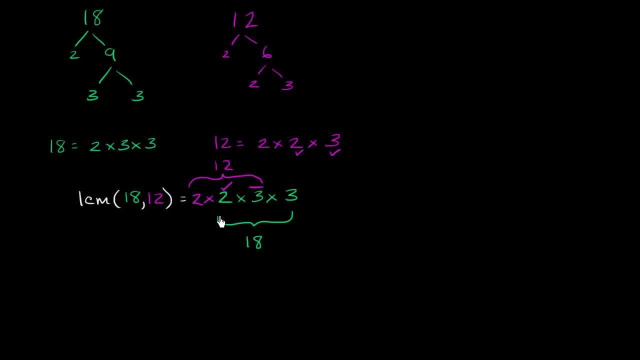 And it has a 2 times 3 times 3, or an 18 in it. So this right over here is the least common multiple of 18 and 12.. If we multiply it out, so 2 times 2 is 4.. 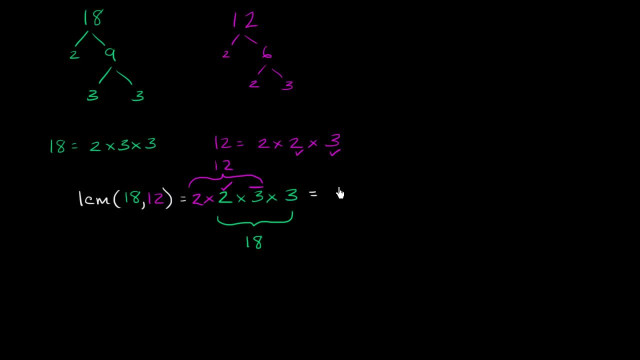 4 times 3 is 12.. 12 times 3 is equal to 36.. And we are done Now. the other way you could have done it is what I would say, just the brute force method of just looking at the multiples of these numbers. 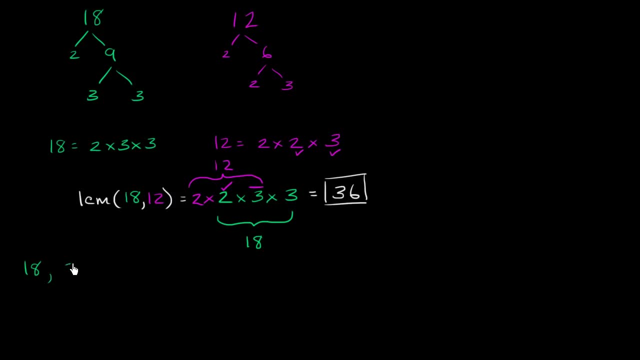 You would say: well, let's see, the multiples of 18 are 18,, 36,, and I could keep going higher and higher, 54. And I could keep going, And the multiples of 12 are 12,, 24,, 36.. 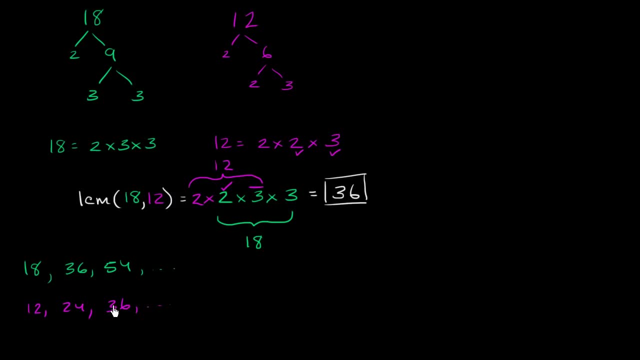 And immediately I say: well, I don't have to go any further. I already found a multiple of both. And this is the smallest multiple of both: It is 36.. You might say, hey, why would I ever do this one right over here as opposed to this one?